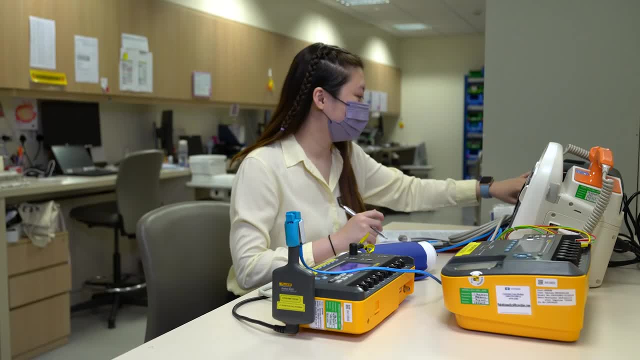 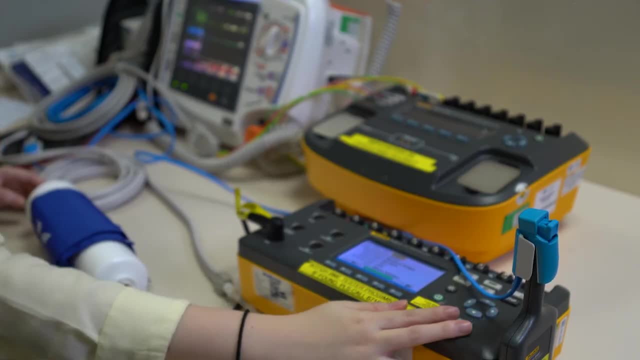 We do preventive maintenance for most equipments as they have their scheduled maintenance that is planned in advance to ensure that the medical devices are working properly. When the user encounters an issue, they will first have to contact us. If the issue is too complicated, we will then contact the hospital. 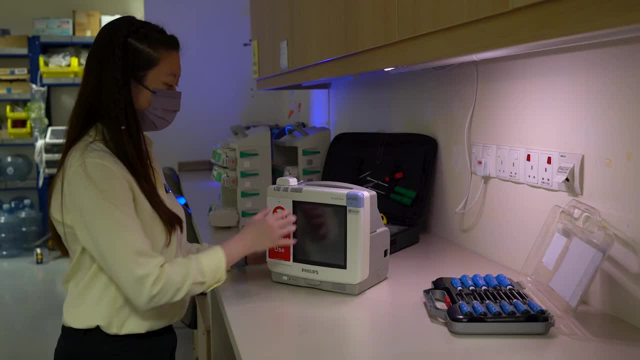 If the issue is too complicated, we will then contact the hospital. If the issue is too complicated, we will then contact the hospital. We will then have to go on site to rectify it. The repairs can range from just changing accessories to opening up what you need. 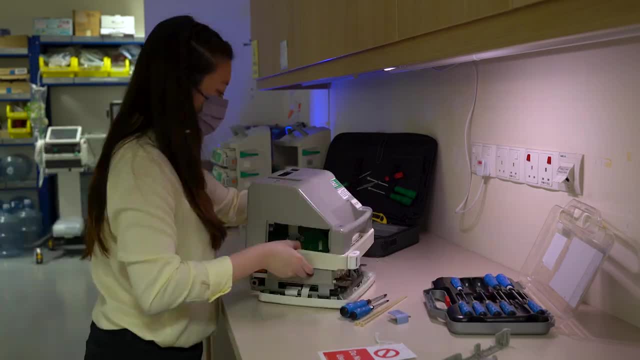 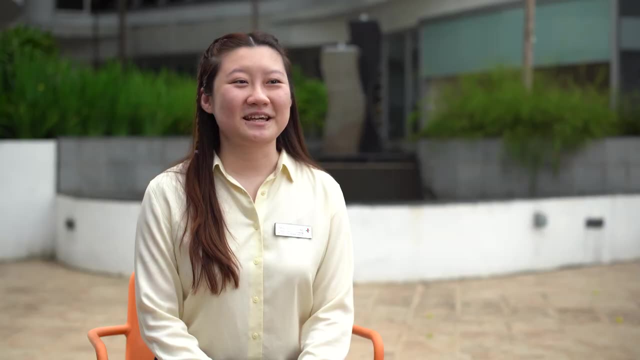 So for the accessories you can do it on-site, but for the repairs we have to bring it back to the workshop. If we cannot fix the device at our workshop, we will then have to contact the vendor and oversee the repair from there. My colleagues and I do have to be on standby after working hours. 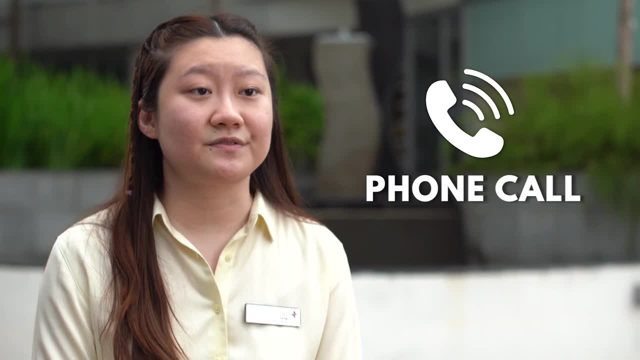 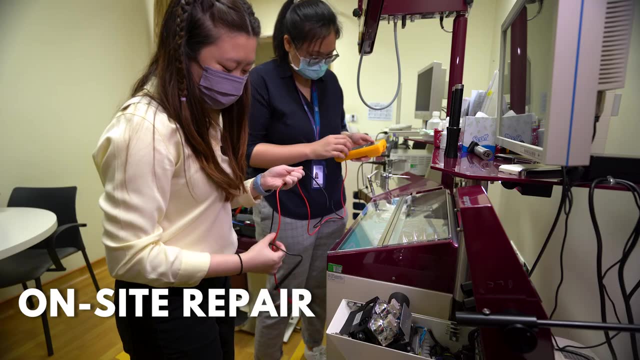 When we receive a phone call from the users, we will first try to troubleshoot the issue over the phone, rectify the issue over the phone. then we have to come down on site, even though it's in the night. Something that people aren't aware of is that we do have to do paperwork. 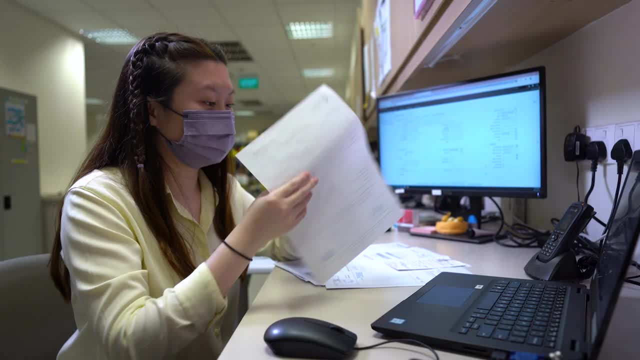 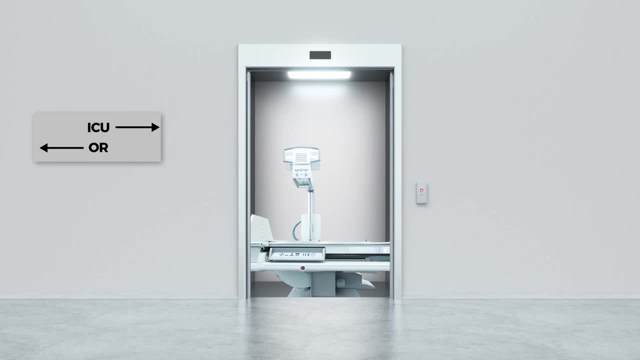 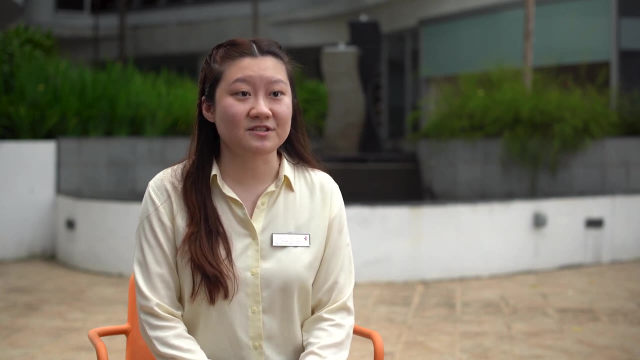 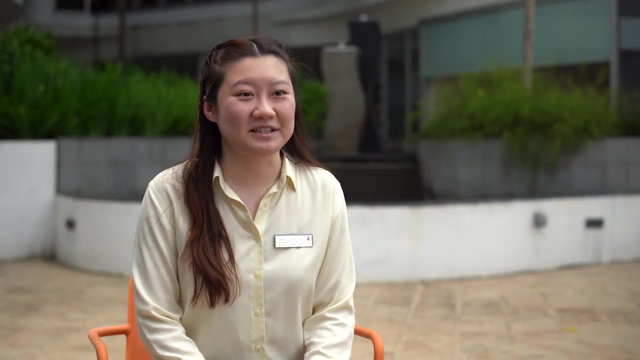 Sometimes we do more paperwork than hands-on repair. One memorable incident that I can remember is that when a portable x-ray got stuck at lift lobby, It was a stressful situation for me, as the lift was being used for patient transfer, So we had to use extension power cords to try to jumpstart the whole machine. 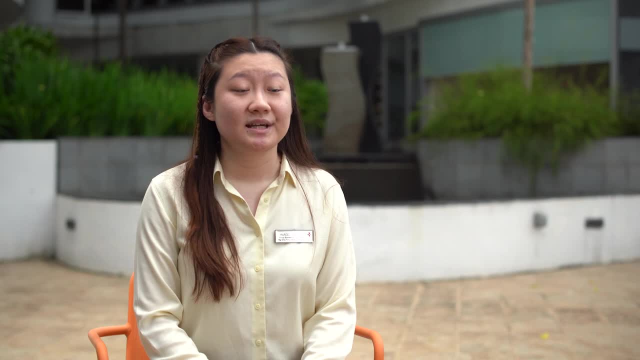 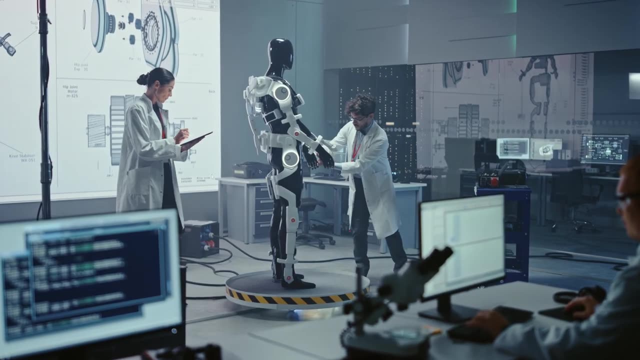 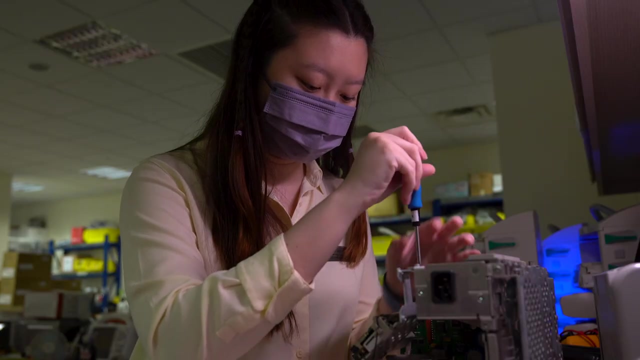 Not a lot of people know what biomedical engineers do, as they think that engineering it means that we are doing with large equipment in the factories, but in fact we only deal with smaller components, as they always assume that only men can be doing all this, but actually we have a lot of female staff. 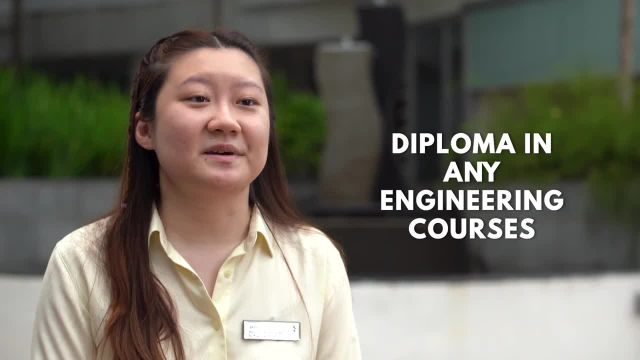 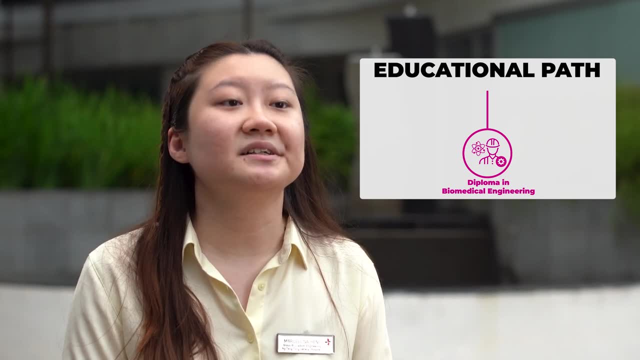 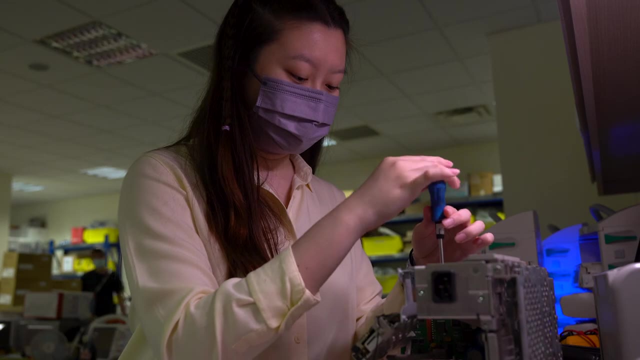 You will need a diploma in engineering to work as a biomedical engineer. I enrolled in the diploma in biomedical engineering, so in my diploma I learned about this career. Engineering is an important skill to have, as we need to know various medical devices. but don't worry, it will be all learned on the job. 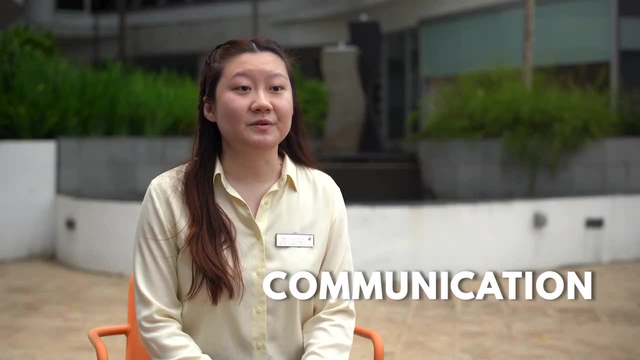 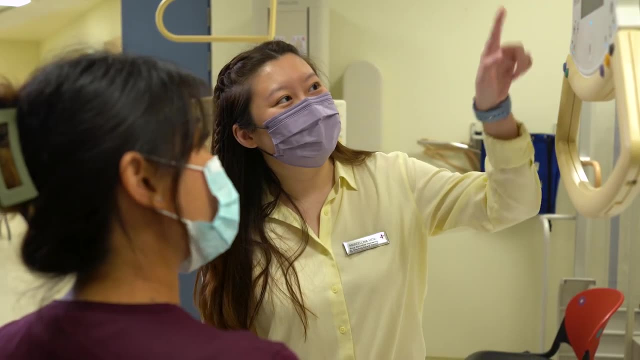 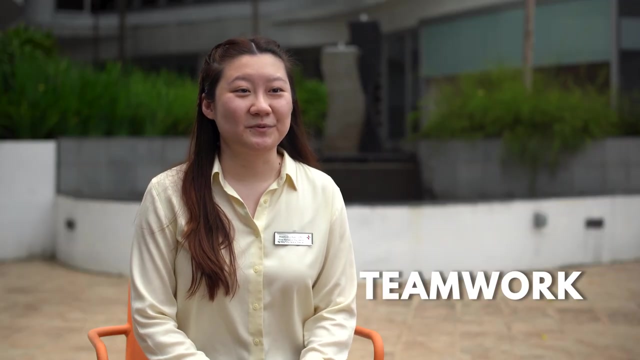 Complication is a very important skill to have as we deal with doctors and nurses on daily basis. There are typically very busy and when we are able to catch their time we need to listen and decipher the issues they are encountering with. Teamwork is important, as we have to work with our team internally and also across departments.